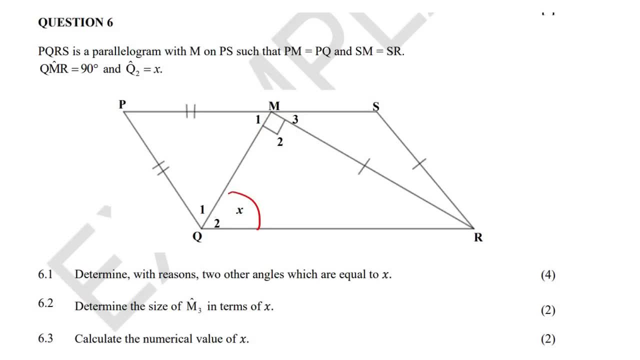 is equal to X. Okay, so that's X over there Now for four marks. it says: determine with reasons two other angles also equal to X. So straight away, we know that this is a parallelogram. So that means that these two sides are parallel. So you see, there's an alternating angle over. 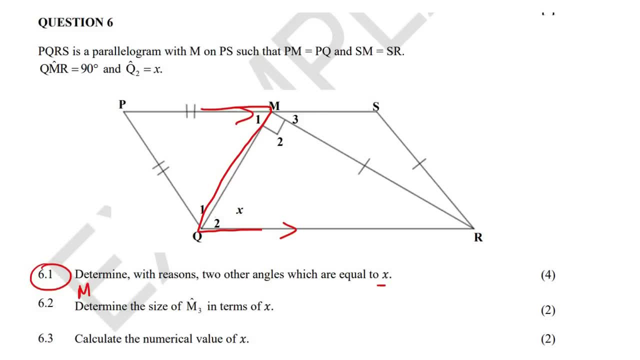 there. So we could say that M1, that's the first one. Why? Because of alternating angles. So you say alt angles, like that, And that is because PS was parallel to QR. You could also say PM, it doesn't matter, But that's fine. So that's M1. And then we need one other. So let's go. 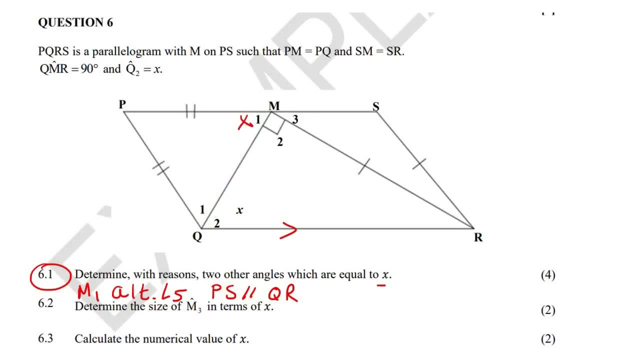 fill that in as X over there. Now have a look at this triangle. It's an isosceles triangle because these two are the same. So when you have an isosceles triangle where two sides have the same length, then the angles- two of the angles- are also going to be the same. How do I know which? 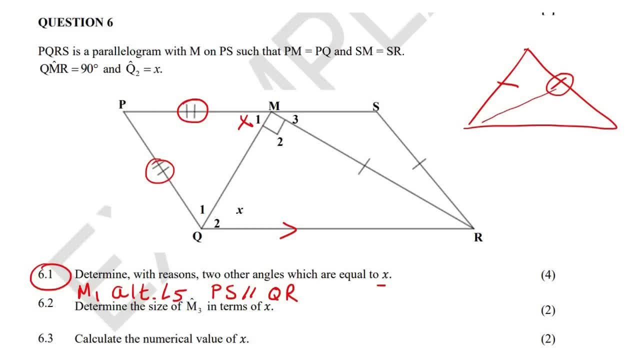 angles. Well, you take this line and you just extend it to the opposite angle, And so these two angles would be the same. So if you take this line and you extend it there, and you take this line and you extend it to the opposite angle, and you extend it to the opposite angle and you 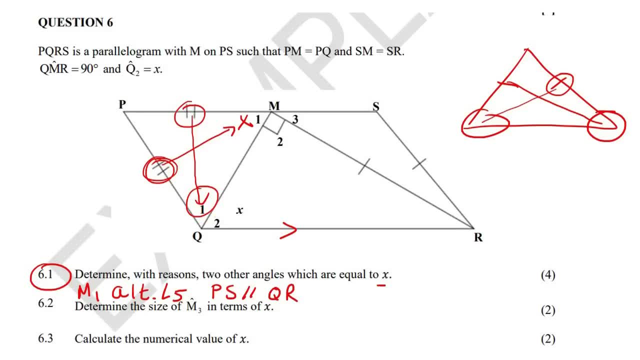 extend it there, then those two are the same. So the other one would be angle Q1.. And that's just because they are the angles opposite equal sides. You're not going to say isosceles triangle. I think in the IEB curriculum that's okay, But in the CAPS curriculum you don't say isosceles. 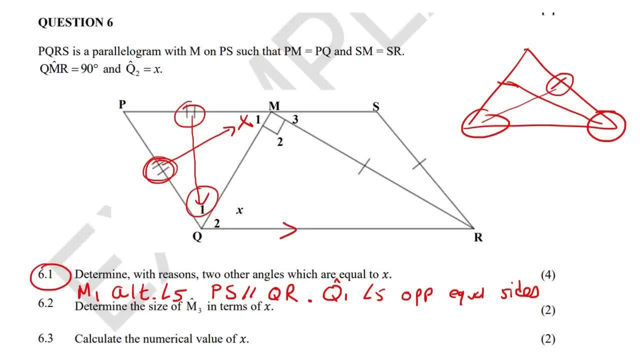 triangle. you say angles opposite equal sides, So let's go put an X there as well. So there's an X there and an X there. Okay, so we've done that one. Now this question says: determine the size of M3 in terms of X, the size of M3. Okay, Well, if you look at M3, we can know that it we know that. 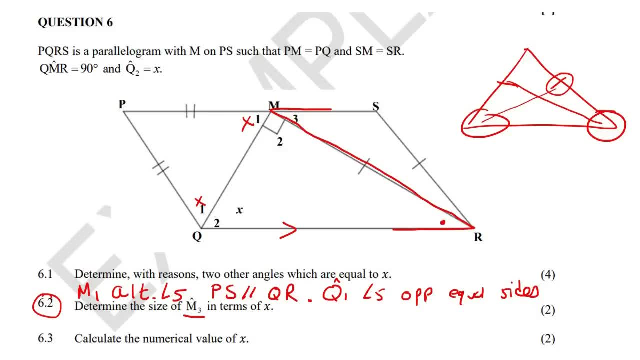 it alternates with this angle over here, right? So, and then we know we can work this angle out, because in this triangle we can use some of the angles in a triangle to calculate this angle over here. So we could say that angle QRM, don't just say angle R, because that could be the whole thing. 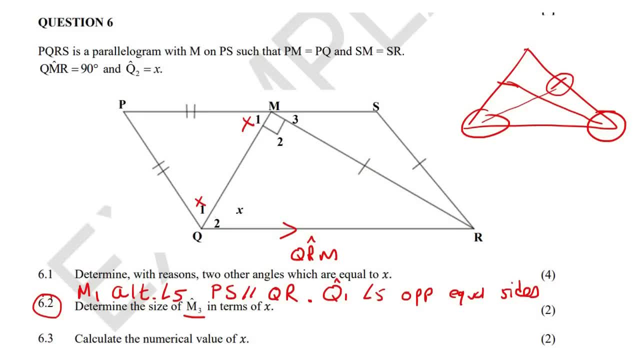 So say QRM. or you could say MRQ is equal to 180 minus 90 minus X, right, And that's just because of the sum of angles in a triangle. or you could just say some angles, triangle. And so if you had to work, 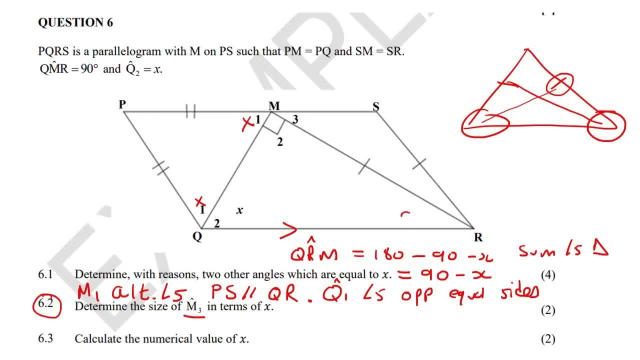 that out, you're going to end up with 90 minus X. So this angle here is 90 minus X, And then, because of alternating, M3 would also be equal to that. So we can then say, therefore, or first: 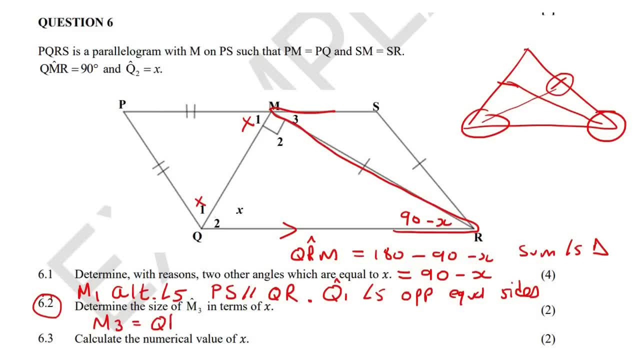 let's say M3 is also going to be equal to QRM, And that's because of alt angles, And that is because the line MS is parallel to QR, And so therefore, angle M3 is going to be equal to 90 minus X, And so let's just go full that in 90. 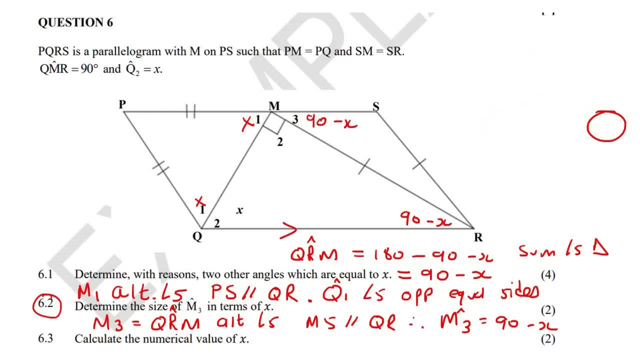 minus X. But now I was checking on the memo, they you could do it in a different way And you actually might get a different answer. So the other way that you could have done this is okay. so that's, that's the one way that you could have done. 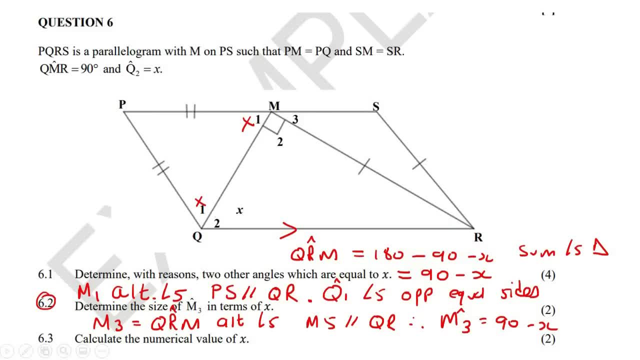 6.2.. But the other way that you could have done it is, for example, we know that if you have a parallelogram, okay, the opposite angles are equal. Okay, so if we know that this is a parallelogram, 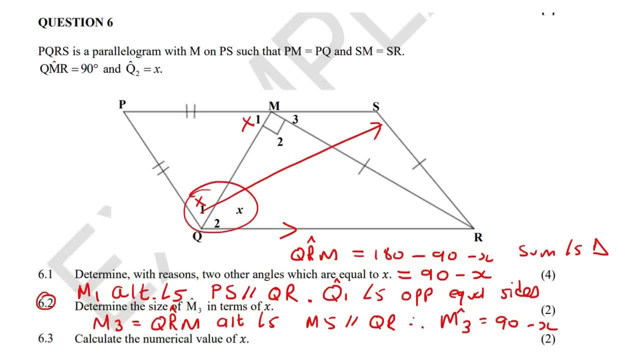 so then the opposite angles are equal. So these two, this angle and this angle, must be the same. So this whole angle is 2x. So we could say that angle S is equal to angle Q1 plus angle Q2.. And your reason for that would be: 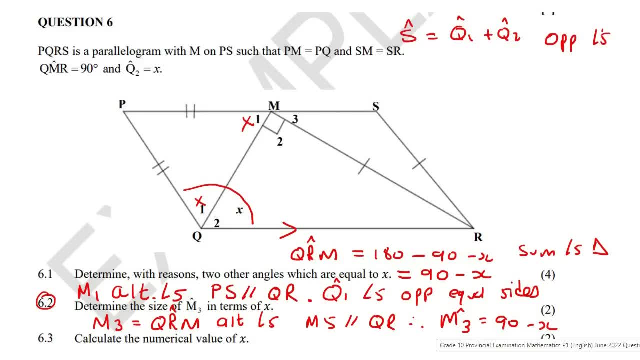 opposite angles of a parallelogram. Okay, well, some teachers write parallelogram like that, So so then that means that angle S is going to be 2x. So this is 2x. But now here in this triangle, 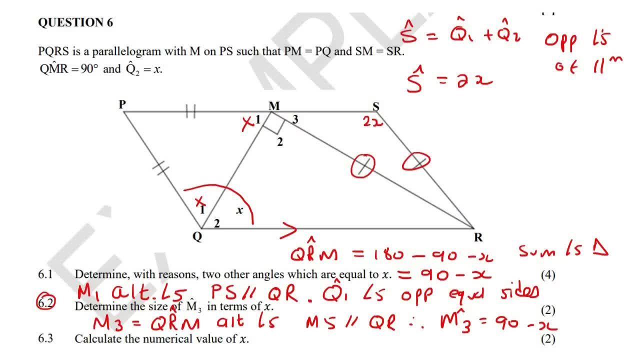 we have another isosceles, because these two are the same. So remember what you do. you take your line and you, you go to the opposite angle. So you can't go to that angle And you can't go to. 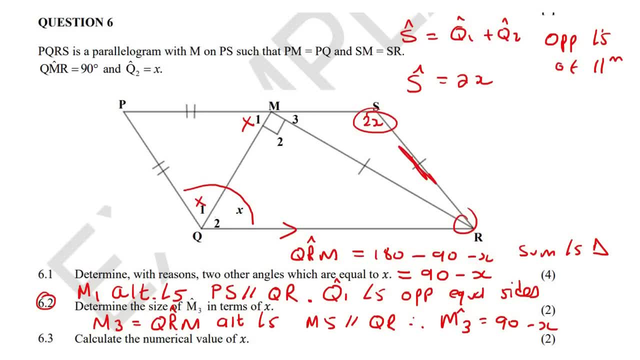 that angle, because those are, those two angles are next to this line. So you go to the other angle, which is this one over here And then this line. you wouldn't go to that angle. And you wouldn't go to that angle because those two angles are.